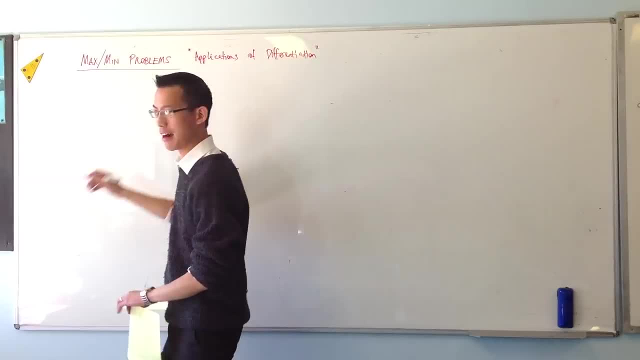 So what I'd like you to jot down first is: I'm going to actually give you the wording of the question. we'll talk through it, okay. So a comet Passing by Earth? So we're going to be thinking about distances, okay? 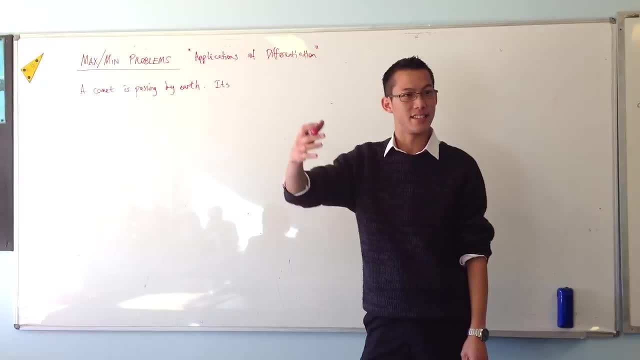 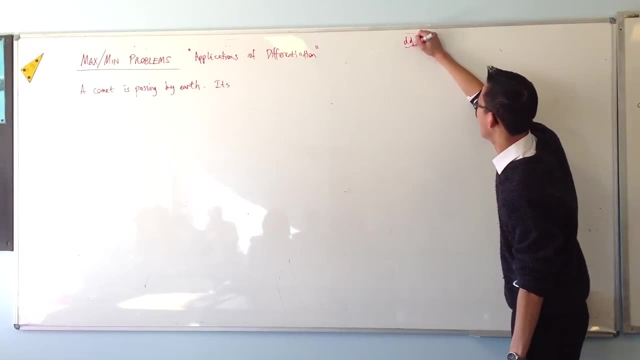 Because it's distances. you might think we would usually say: you know, let distance be d or something like that, But I'm actually going to say rather than d, because then we're going to have like dd on dt, which is a bit confusing. 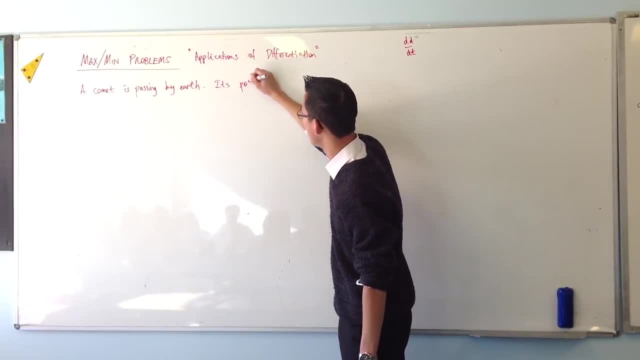 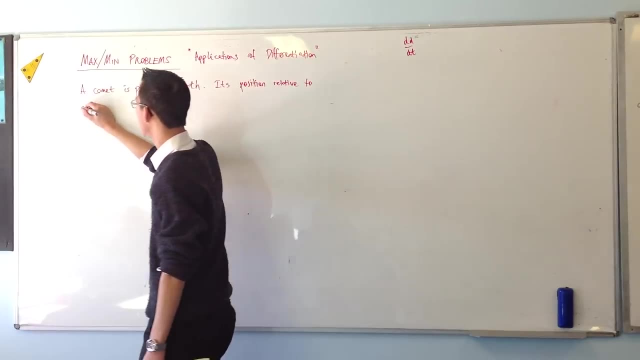 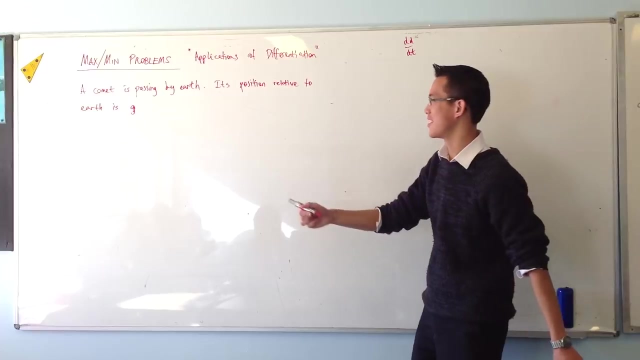 So I'm going to call it p for position. okay, So it's position. So it's position relative to Earth. Could you use s for displacement? Yeah, I could use s for displacement. It's just as- yeah, I mean it's just as random as p in some ways. 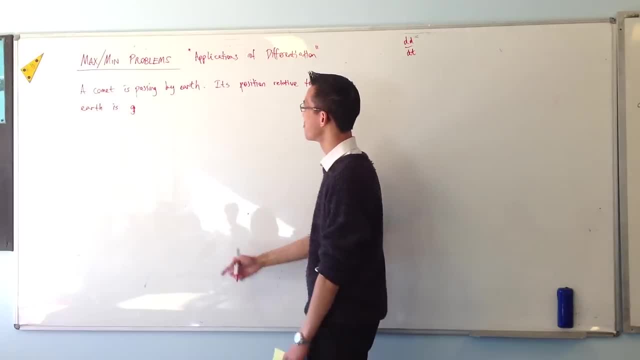 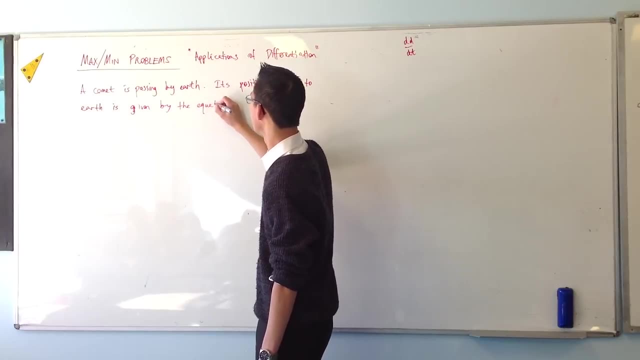 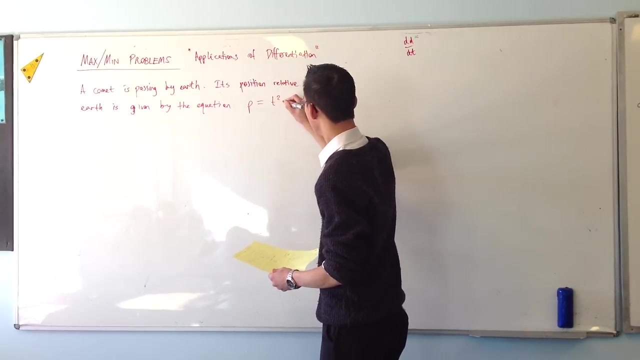 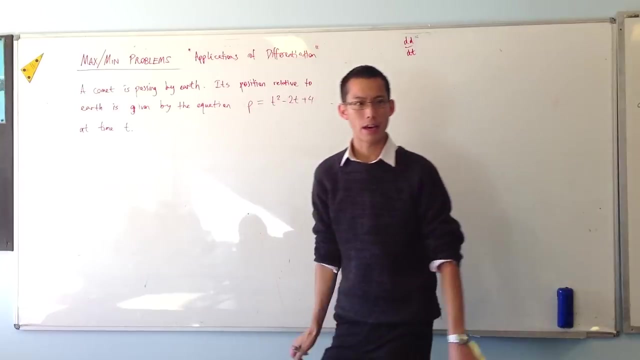 Because, like s for displacement anyway, It's position relative to Earth is given by the equation p equals. Now, I can't, I can't with one, Let's go with this. Okay, It's position relative to Earth is given by the equation blah, blah, blah. 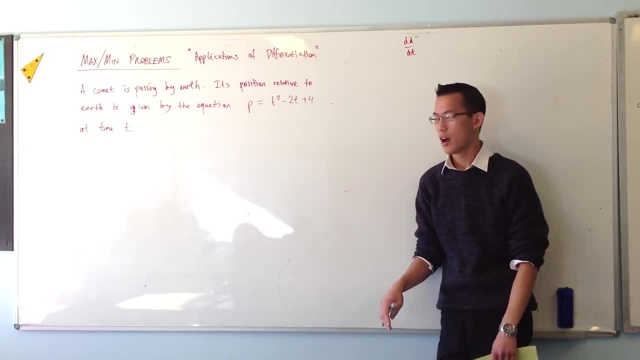 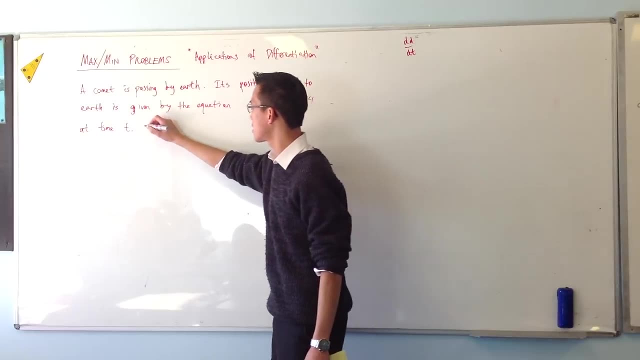 Now, because this is a it's a problem solving thing, right. Usually we're used to derivatives and all that kind of thing having no units on them, But these obviously have to have units, okay, So let's say p is in. 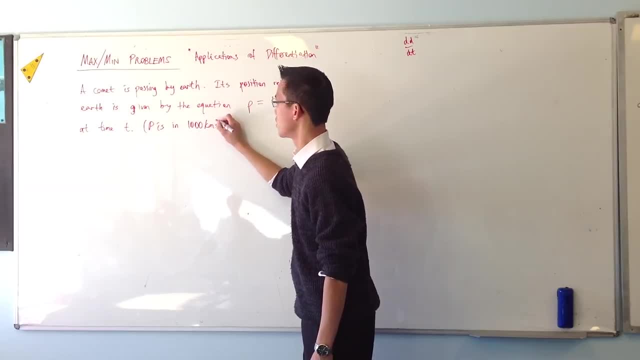 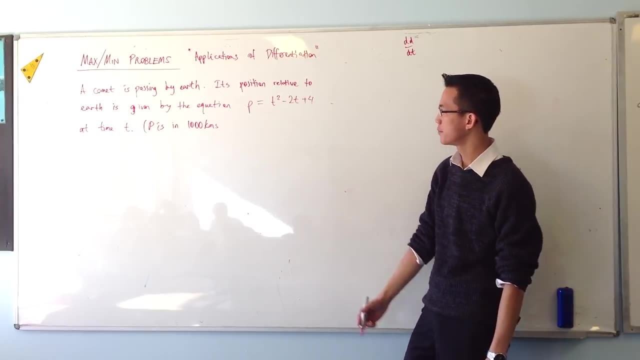 thousands of kilometers. Okay. So if p was one, okay, That means the comet is a thousand kilometers away, p is two, two thousand kilometers away, etc. Okay, And t is in days. Okay, So it might be hours, minutes, seconds, doesn't matter. 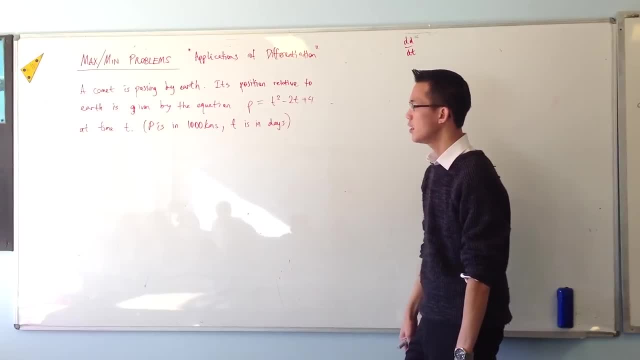 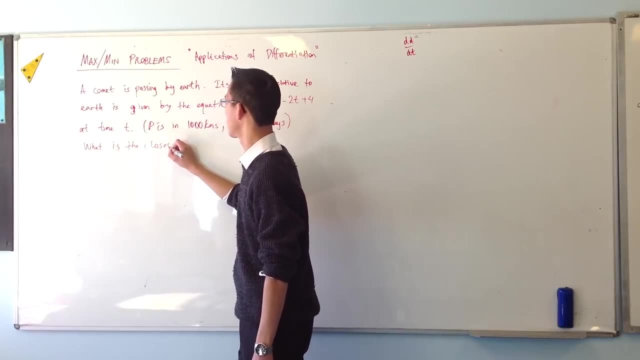 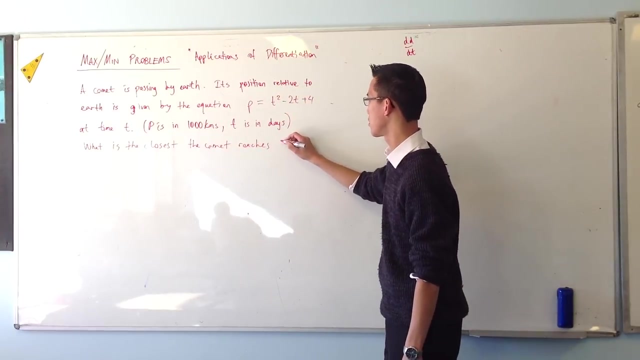 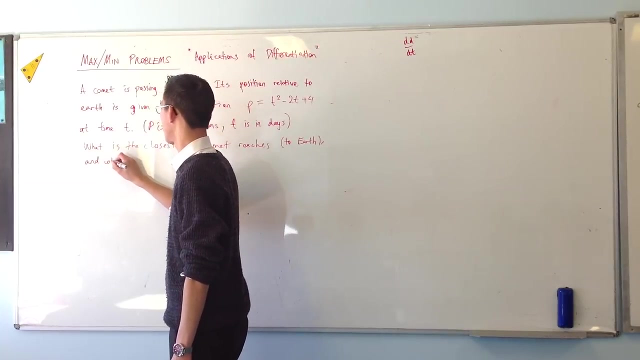 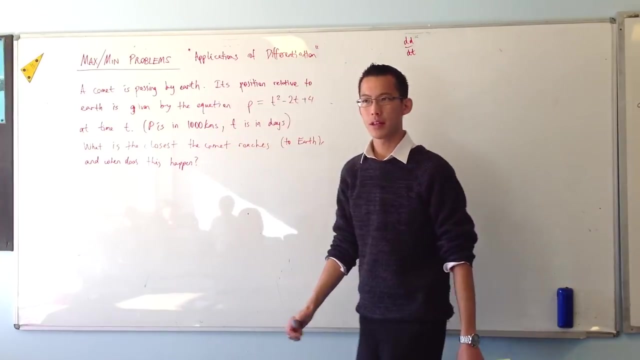 So long as we pay attention to what they are. So the question is, what is the closest the comet reaches closest to us, and when does it happen? Okay, Now, this is pretty standard for a maximum problem. okay, You've got your scenario. 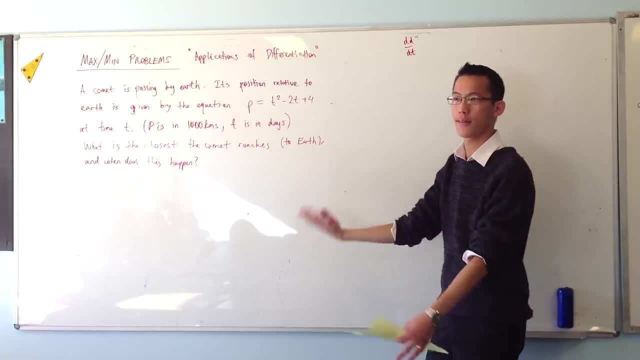 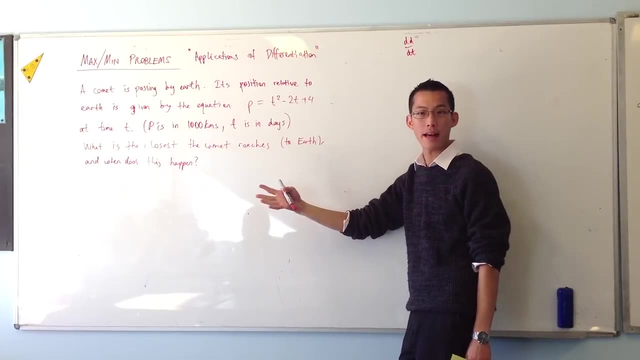 They'll give you some kind of equation which tells you about what governs the scenario, and then they'll pose you a question based on that: okay, And what our job is is to interpret this and think about: okay, what maths am I going to have to do to solve it? 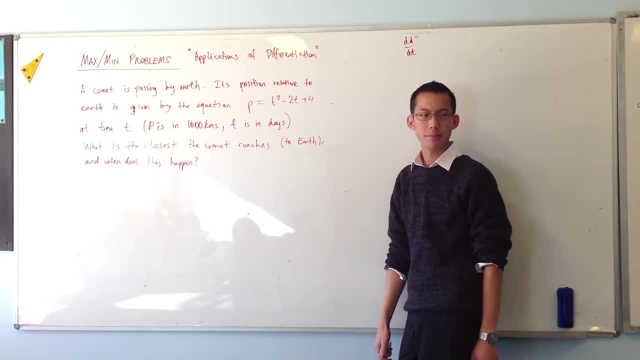 Yeah, Do they always give you equations? Aren't there problems where they won't give you- That's right. So I'm starting off nice and simple, okay, And we're even starting with a really simple equation as well. Yes, 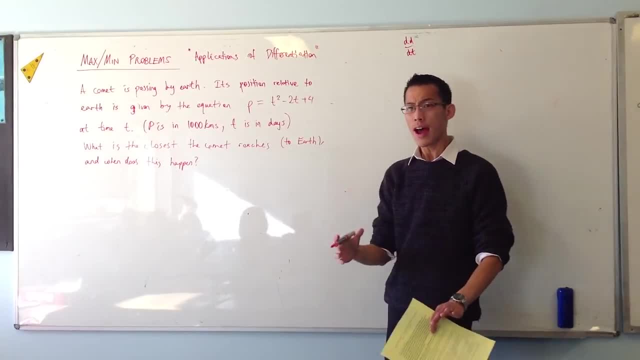 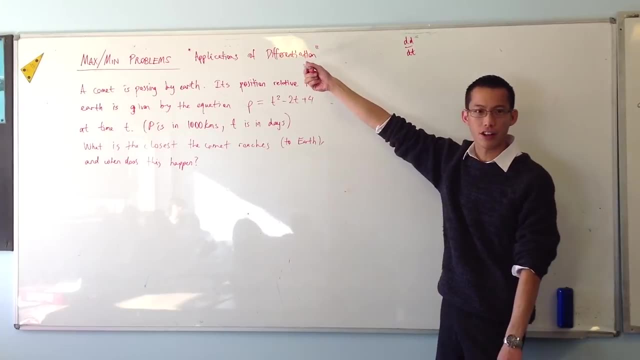 We'll get into the complexities as time passes. Okay, Right now, how are we going to do this? My first advice, before we actually apply any- uh, you know- actual calculus to it is: can we just get a look at what this thing is doing? 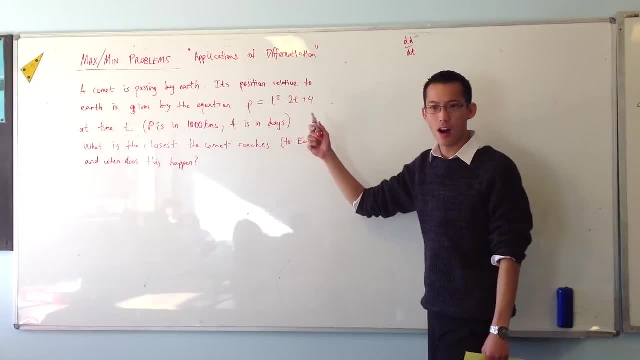 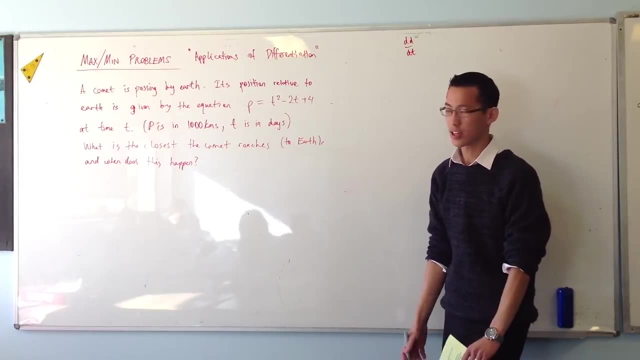 What's it behaving like, okay? So this thing here, we can graph this, okay, And that'll show us, uh, how's this comet behaving, and then we can start to apply problem solving to it. Okay, Some people will start doing the numbers first in the equations, but I think this way will guide what kind of things you do. 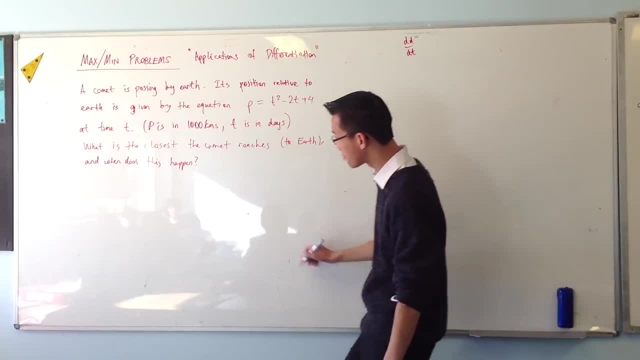 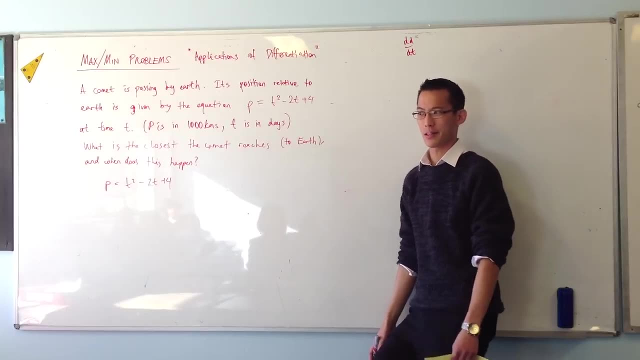 Okay, So p equals t squared minus 2t plus 4.. We can graph this. What would be the first thing that you do? To work out what it is, To work out what it looks like as a graph. Say it again. 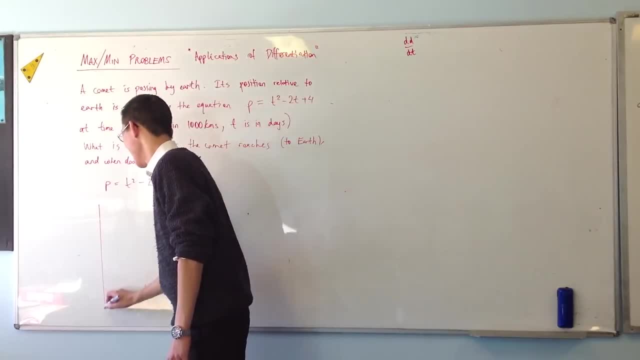 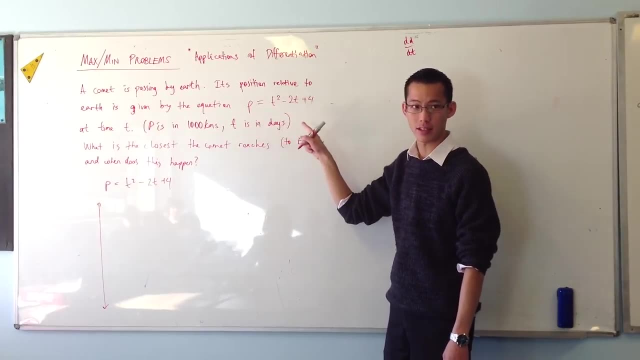 Axes, Axes, okay. Well, let's draw it Now before I go on. usually we're used to a y and an x axis, right, But I don't have y's or x's here, So p is going to be my vertical axis. 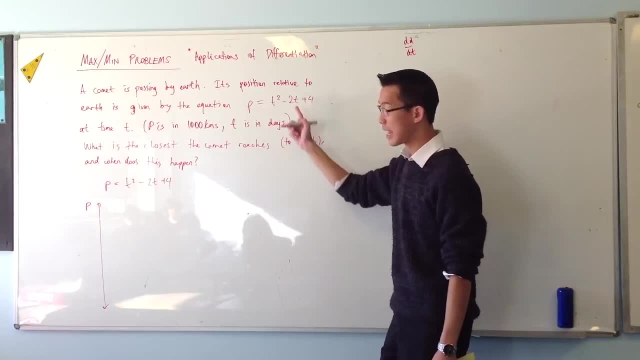 P Right. So that's the distance And t is going to be my horizontal axis. Now I will say for this question- and this is most often the case- that t is specified, it must be positive, but sometimes it's not. 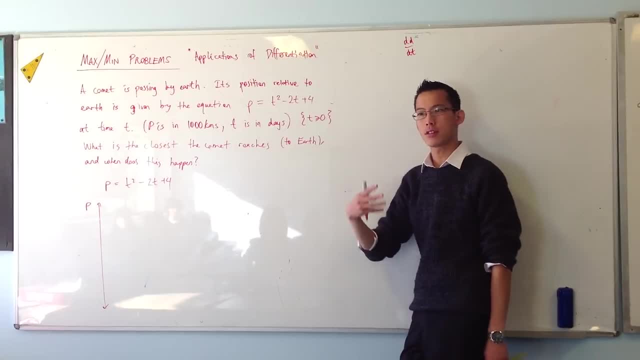 Okay, For instance, the question might say: t equals 0. is 12 noon, 12 noon, Right, And therefore negative values for t are meaningful. Right, Like t is minus 5, might be like 7am or something like that. 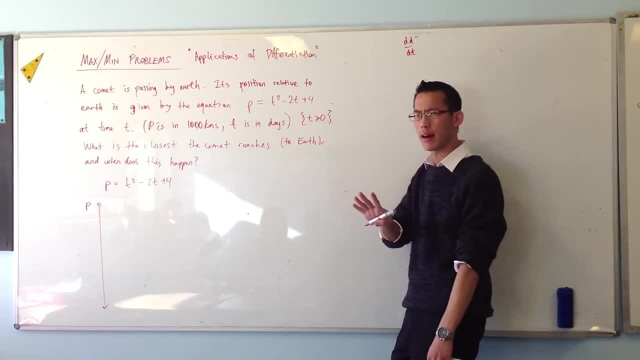 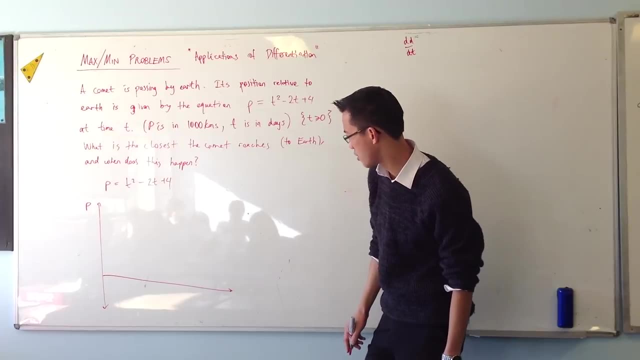 Okay, So just watch out. This is the? u case, but it's not always. Alright. Now, because it's the case here, I'm just going to draw the positive side of the t axis. That is such a not straight line, but 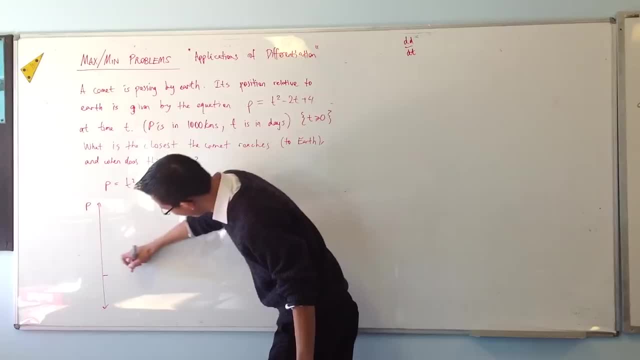 Close. I'm going to fix it. I'm going to fix it because There's a grid on this board. I don't know if you can see it from where you are, but it makes it really, It's really faint. 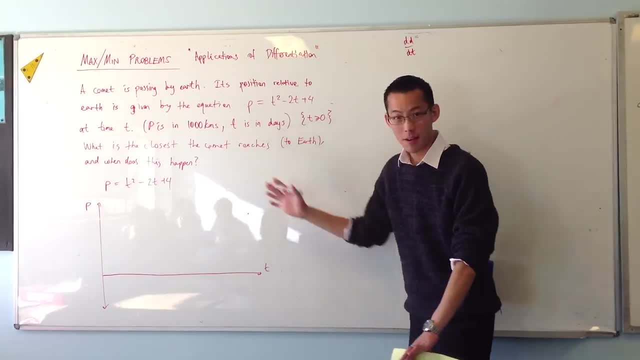 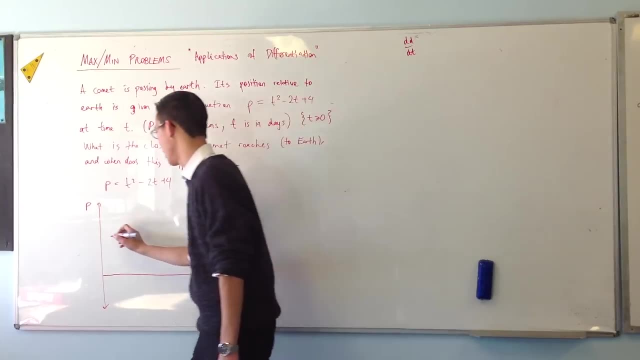 It's quite faint, isn't it? Okay, So there's my p and my t axis. Now, before I do anything, I already know that the p intercept is 4.. Okay, So I'm going to stick that there. 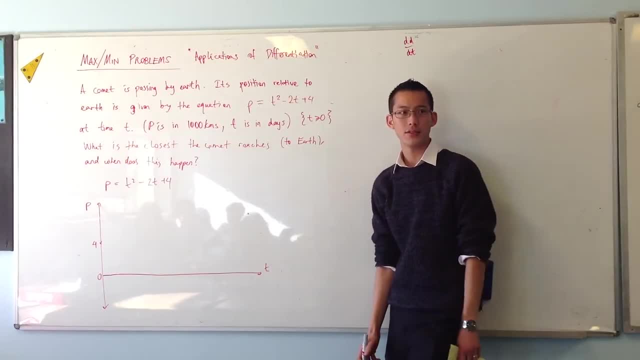 There's 0. Alright, But what does the rest of it look like? How are you going to work it out? Well, it's going to be concave up, Okay. So I can see that because I've got a positive coefficient of t. 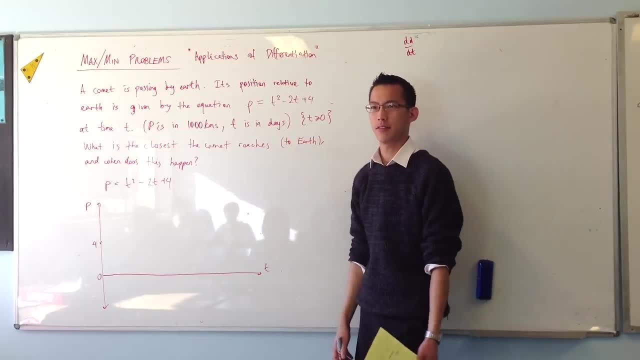 T squared. sorry, But what else do I want to know about it? Okay, Intercept is the first place to go. Okay, However, you look at it and you're like: okay, you don't have to do this every time. 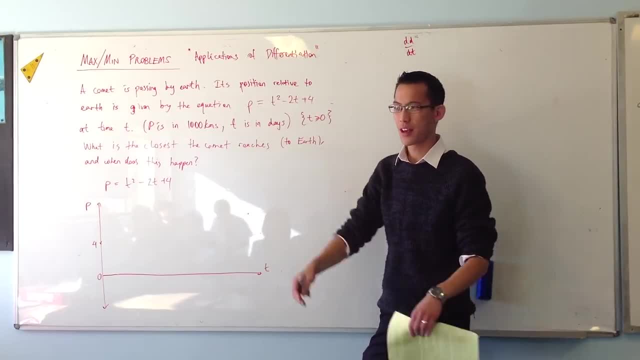 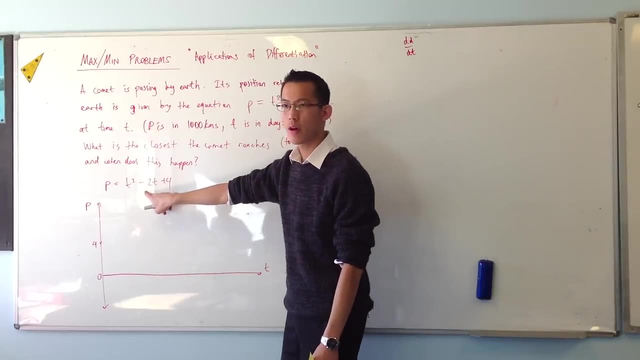 but I've thought of this question in advance, so I already know. You can know what kind of intercepts you're going to have by looking at the description Right Discriminant B squared minus 4ac. Now that looks to me like 4 minus 16, minus 12.. 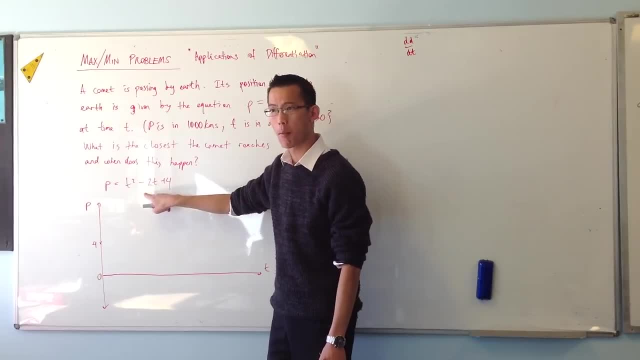 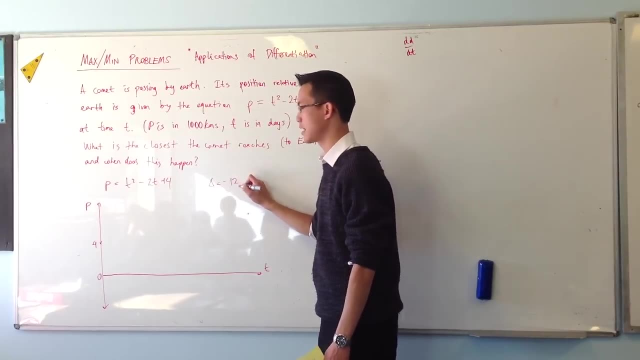 Okay. So if the discriminant is negative, what does that tell you? No exit of cells. Okay, So it's concave up. It's going to do something like: well, I don't even know where the axis of symmetry is. 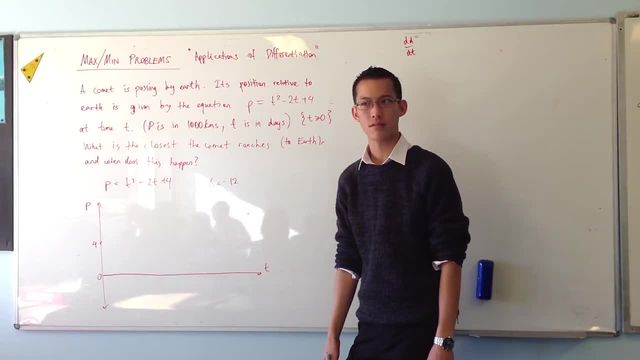 Right, So you're going to have to do something like this. Okay, Sorry, No, Yeah, It's a good thing. Yeah, Thumbs up. Okay, So this is good. Right, I don't have any roots. 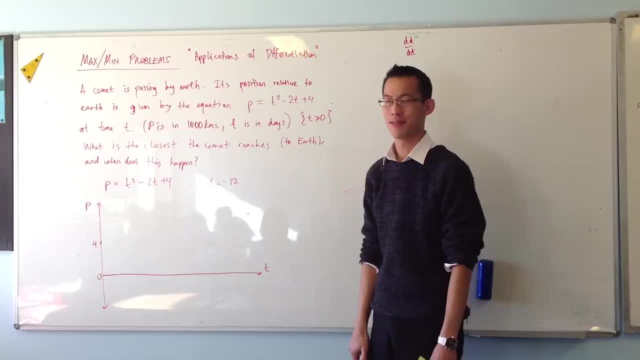 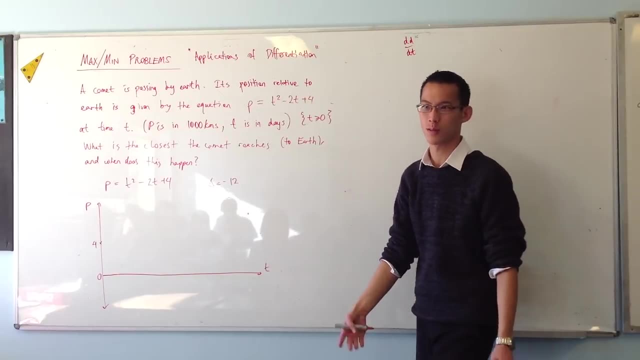 So how else am I going to work out what this looks like? What would you do? Submit values. Submit values. I could submit values. What's an important feature of the graph? The vertex. Okay, The vertex. That'll be useful for us. 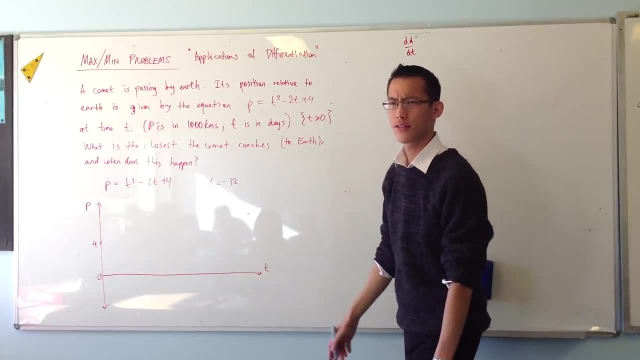 And in fact not just is it useful to know what it looks like, but it's kind of useful to the question as well: How do you work out the vertex axis of symmetry? Okay, So the axis is minus b on 2a. 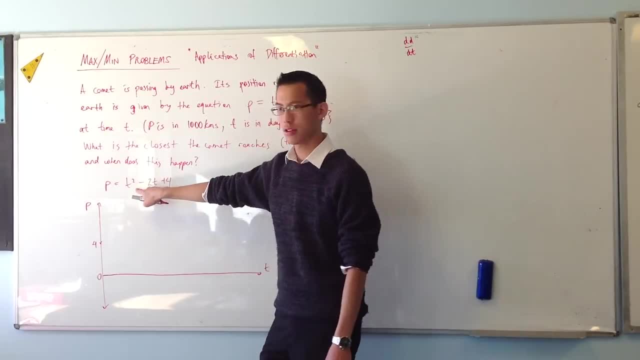 Minus b on 2a, So that's minus 2.. Minus 2.. So positive 2 on 2a, 2 over 2. That's 1.. Okay, So there's my x value. 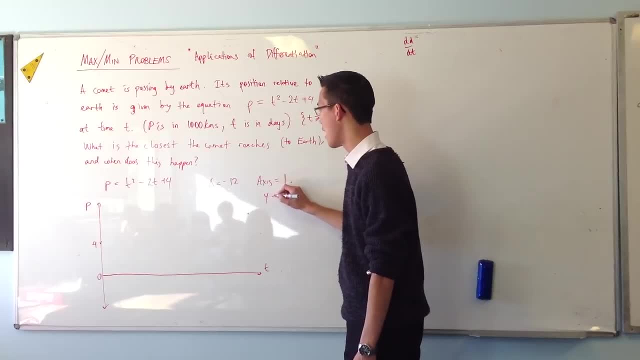 So therefore the y value for that, plug it in 1 minus 2 plus 4.. 1 minus 2 plus 4.. Sounds like 3.. 1, 3.. Okay, So that means that I've got.